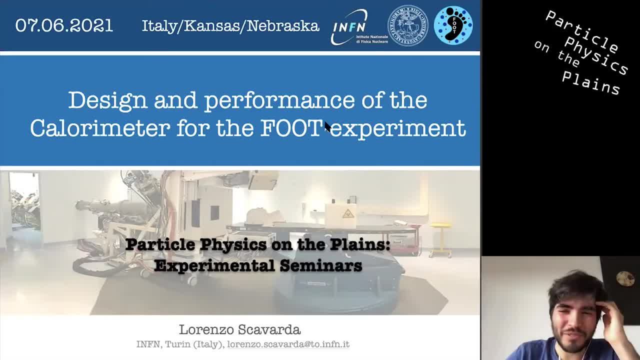 So today I will tell you about the FUT experiment, in particular, about the design and the performances of the calorimeter-optic experiment. As I said, I'm a PhD student of the Turing University in Italy and I'm working for the INFN, the Istituto Nazionale di Fisica Nucleare. 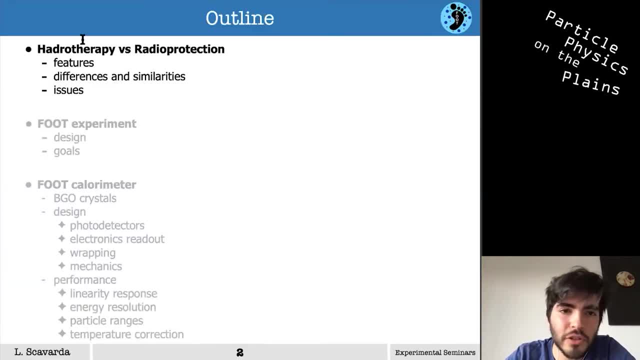 OK, so I decided to split my presentation in three parts. I will start with an introduction, where I will tell you about the topics and about the purpose of my experiment. Then I will speak about the experiment itself And the last part- I will speak about my contribution and the main task of my group inside the collaboration. 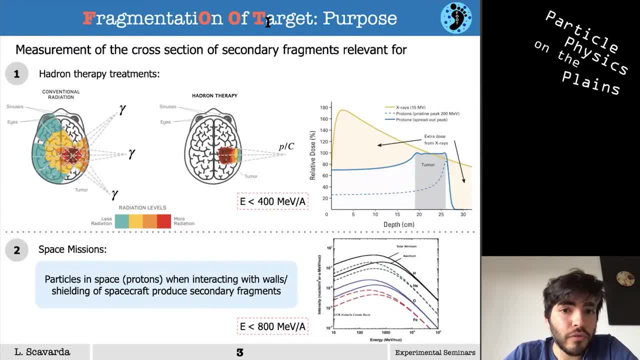 OK. fragmentation of target or FUT. FUT is a nuclear physics experiment and it wants to measure fragmentation, cross-section of secondary fragments created in interaction between a primary beam and a fixed target. These measurements will be relevant for two main topics: for the adrenotherapy and also for the space munitions. 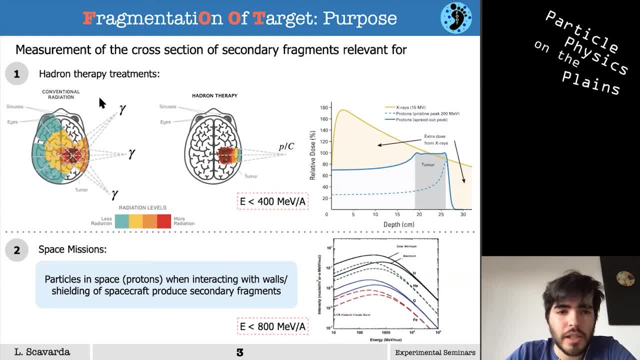 OK, just some words about the adrenotherapy. The adrenotherapy is a kind of radiant therapy, So with conventional radiation, But with the adrenotherapy we will use proton or carbon ions, so adrens, And this approach has a lot of advantages. 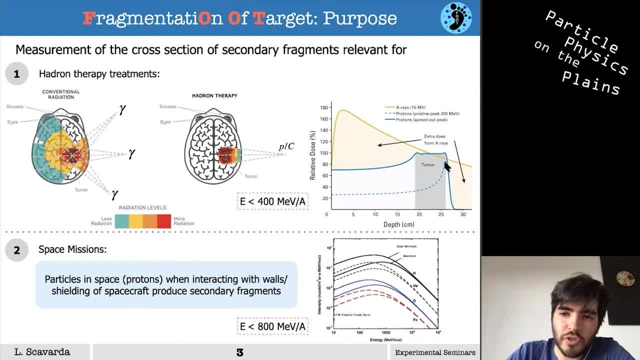 And the main one is the profile of the energy released inside the patient. So, as you can see in this plot with the blue trend, we can see that the energy released in the entry channel, So on the surface of the skin of the patient, we release low energy. 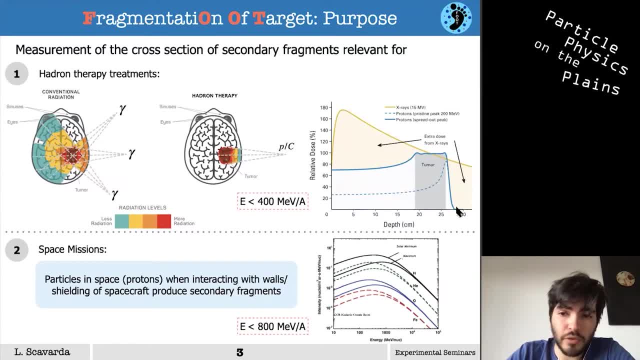 And the maximum of the dose is released where there is the tumor, So inside of the patient, So changing the energy of the primary beam, the treatment particle. we can move this peak, called also Bragg peak, And we can scan on all the surface of the tumor. 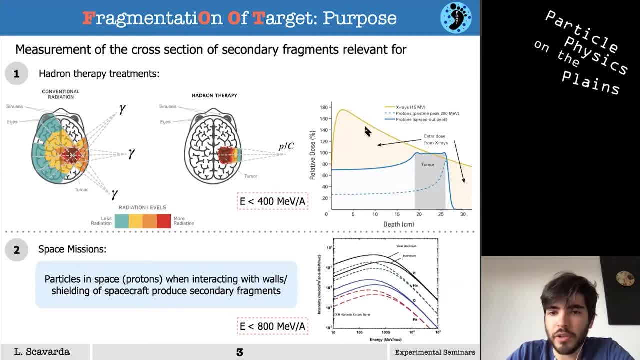 With the radiant therapy. instead, we have a different profile because we have the maximum of the dose in on the surface of the skin. So we can have a lot, of a lot of advantage with this second, with the first approach. But there is there are also some problems with this kind of therapy. 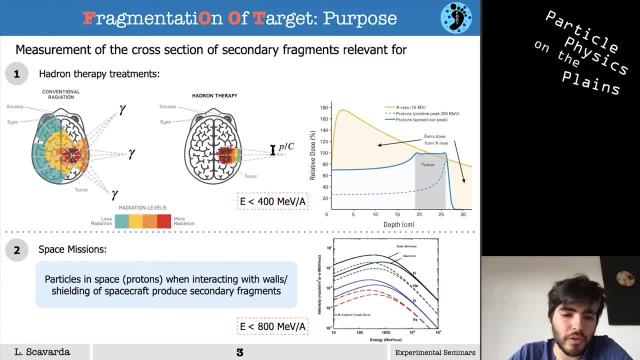 The main one is that this particle, for their natural They, can interact also with the nuclear force, And so when these particles interact with the atom of the human bodies, they can create secondary particles inside the body of the patient, And so the secondary particles can release their energy in some tissues or organ that maybe you want to preserve. 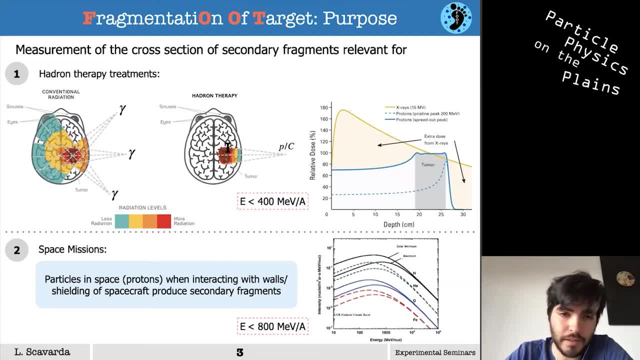 So, in order to improve the treatment, then these treatments, we need to know very well these processes. So we need to measure the cross section of these fragmentation processes Because thanks to these measurements, or better, we can give these measurements to the medical, and the medical can improve the treatment planning system created for each single patient. 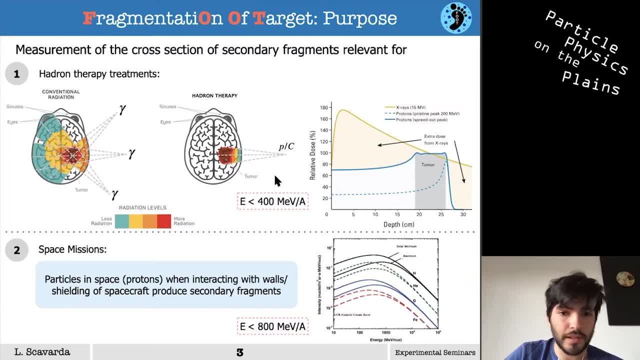 And so they can also improve the treatment itself. But this measurement will be useful also for another topic, as I say, the lightning space missions, because in the space we had similar, Similar effect of the other therapy, because with cosmic, when cosmic rays interact with the walls or shielding of spacecraft, 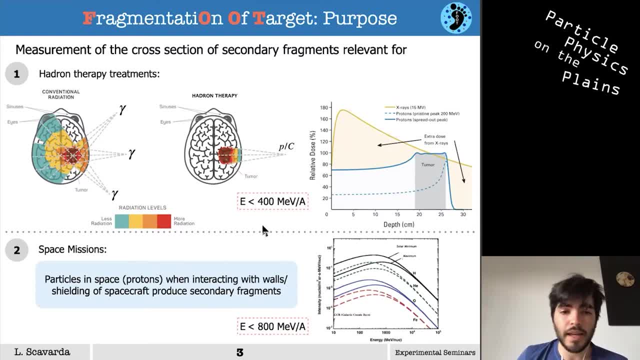 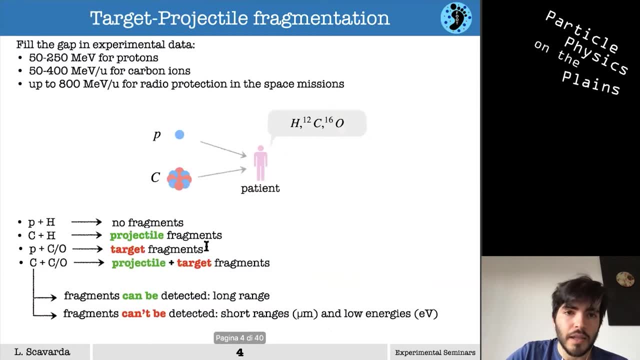 they produce secondary fragments inside the vessel And these secondary fragments will be dangerous both for the astronauts but also for the electronic devices. So my experiment could wants to fill the gap in experimental data of these fragmentation processes in different energy ranges For the proton therapy. 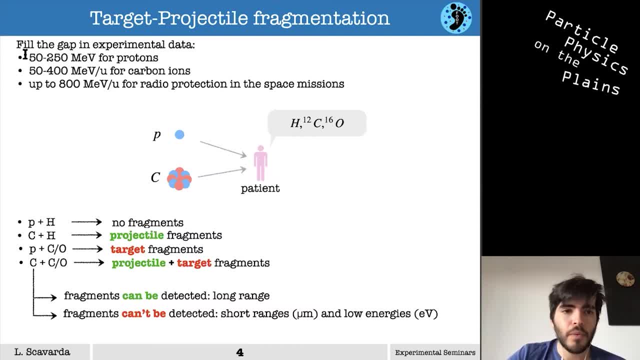 So other therapy with proton beams, We will do measurements in energy range between 50 and 250.. For other therapy with carbon ions, we'll we'll do measurements with the with beams with the range between 50 and 400 per nucleus Instead for the radio protection. 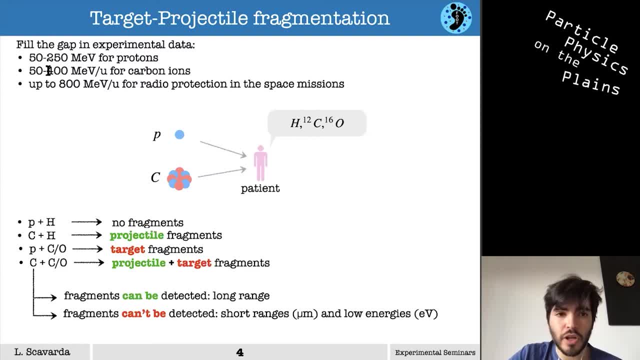 we have to extend the energy range up to 400.. So the idea is to use proton and carbon ions like beams on a target or carbon or oxygen. But there is a problem with this, with this situation, because, for example, if we take protons on carbon or oxygen targets, 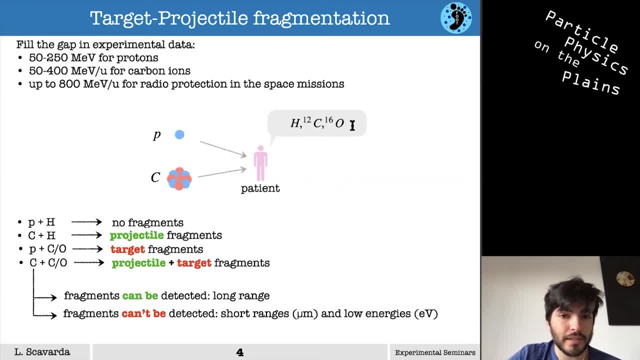 the fragments will born only from the targets and not from the beam, of course. So in these cases the fragments will have very low energies- about some EV- And so they will. they will cross very short ranges- about some micrometers, And so they will be not detectable because they will not escape from the target. 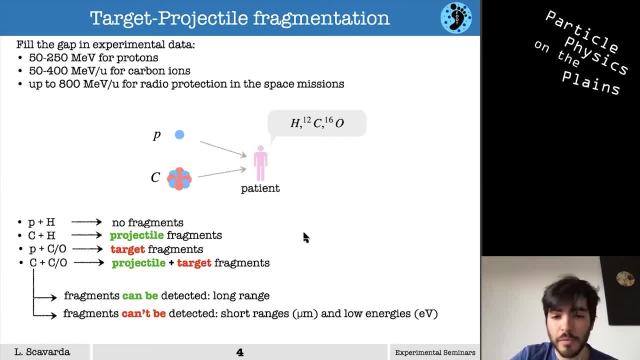 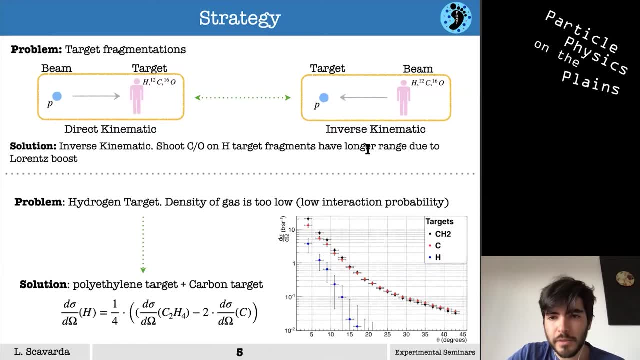 And so we can't. we will be not able to measure the cross section. So the strategy of the food experiment is to work in an inverse kinematics. So instead to use a proton beam on a target of carbon or oxygen, we will work in the opposite reference system. 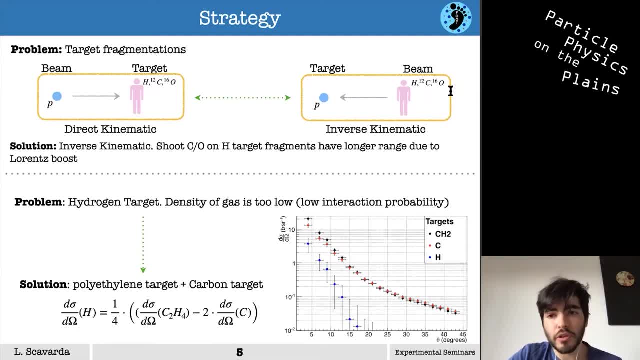 We will use carbon or oxygen beam on a proton target. In this case, the fragments will have longer range due to the Lorentz boost And after the measurement of the cross sections. we can, we, we can come back in the process. We, we can come back in the previous reference system. 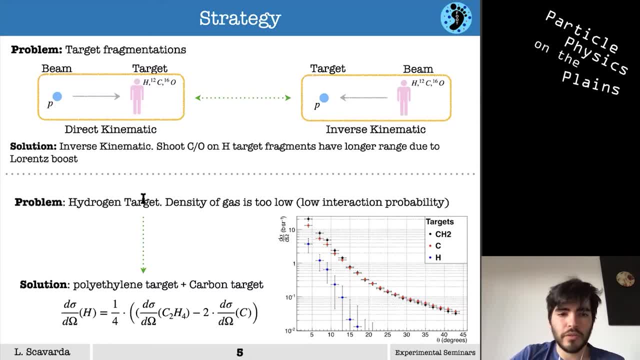 But there is a second problem, because we can't use hydrogen target because the density of the gas is low and also low interaction probability. So we will use a combination of two targets, a polyethylene and a carbon one. From the subtraction of the two cross sections with the two different targets we can find what we need. 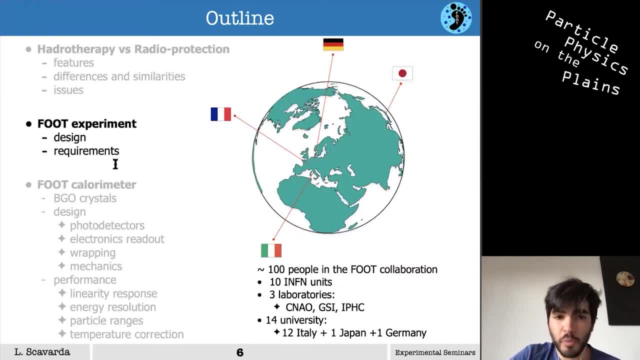 OK, so we can skip to the second part about my experiment, And so I will tell you about the design and the requirements of this experiment. First of all, we are an international collaboration about 100 people, And then the biggest part of this collaboration is in Italy. 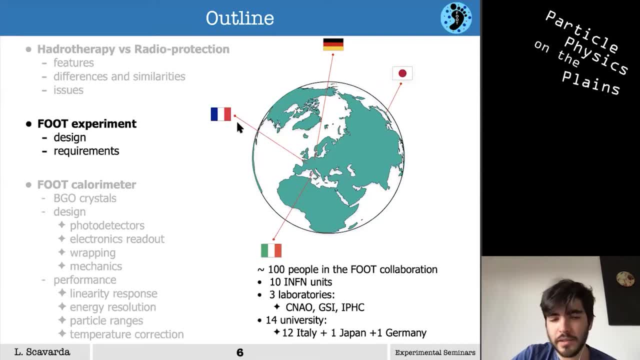 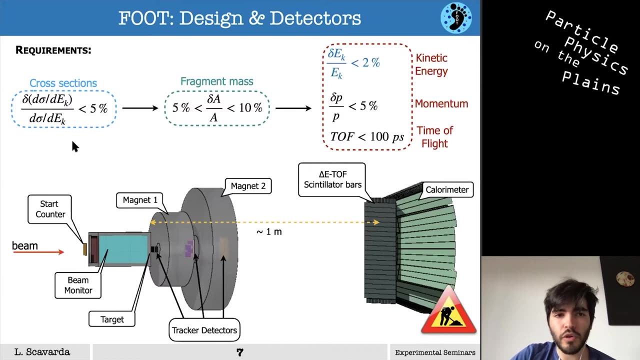 But we have also one group in France in Strasbourg, and a couple of groups in Germany At GSI and in Aachen, and one small group in Japan at Nagoya. OK, as I say, the goal of our experiment is major differential cross section of the fragmentation processes with a resolution below 5%. 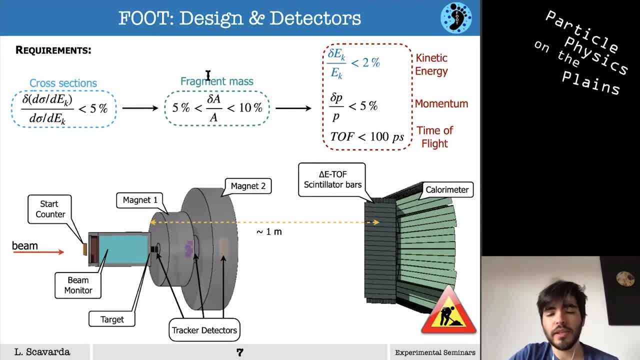 But in order to achieve this value, we need to identify very well the fragments. So we need to measure the mass of the fragments. Here we have the range of the resolution on the mass, But in order to identify the mass of the fragments we need to measure three different quantities. 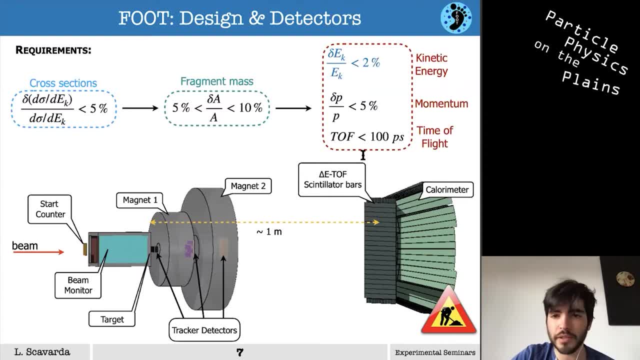 The kinetic energy, the momentum and the time of flight. Combining two by two these quantities, we can calculate the mass in three different ways And thanks to this redundancy measurement, we will be able to exclude the events where the mass is not calculated properly. 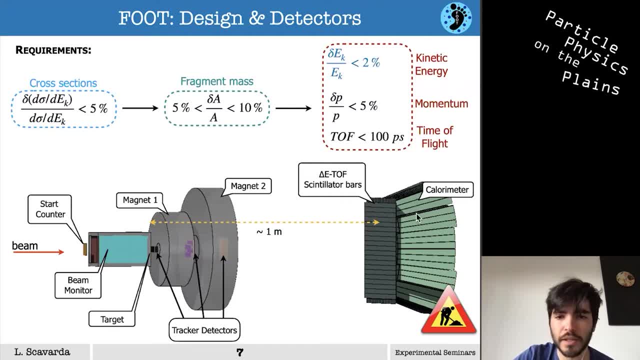 For example, when we create neutron inside the calorimeter. So for these reasons, we've decided to design the foot experiment like in this sketch. We can start from the left to the right. We have the beam, Then we have the star counter. 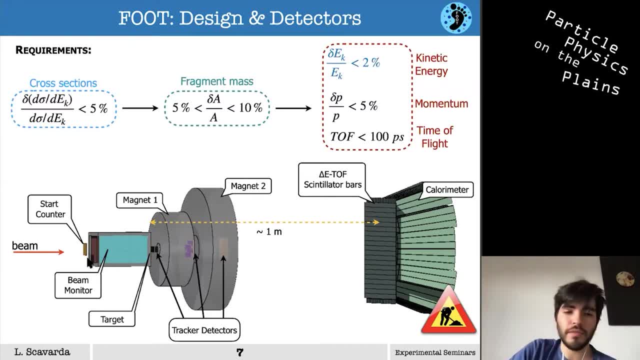 The star counter. Basically it's a plastic scintillator in order to give the trigger to the experiment but also the start of the time of flight. Then we have the beam monitor. Just basically it's a drift chamber just to monitor the position of the beam before the interaction point. 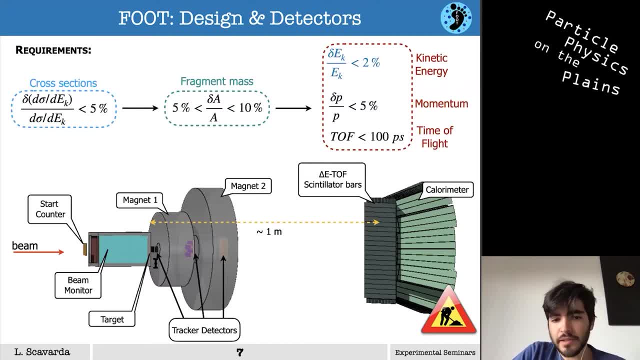 Because after this detector we have the target. After this we have the magnetic spectrometer in order to measure the momentum of the particles, with three different tracker stations. So three different tracker detectors: We have pixel, pixel and microstrip and two magnets. 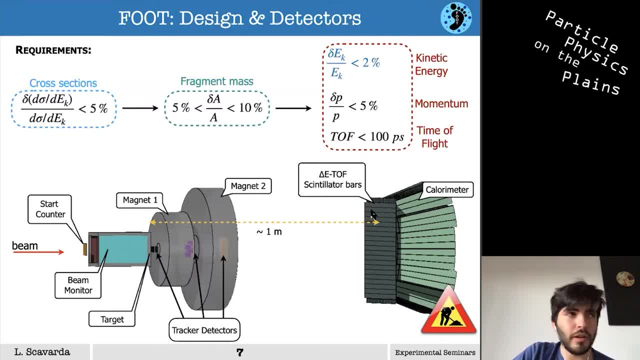 After this, we have the so-called- what we like to call- TOF wall. It's again a plastic scintillator composed with scintillating bars, vertical and horizontal, And thanks to this detector, we can have the stop of the time of flight. 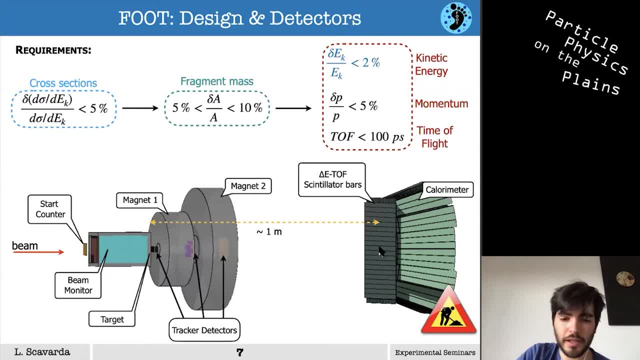 But also the charge of the particles from the energy loss of the particle inside the scintillating bars. The last detector is the calorimeter. Yes, one thing that I want to underline is that the dimension of this experiment is not very big. 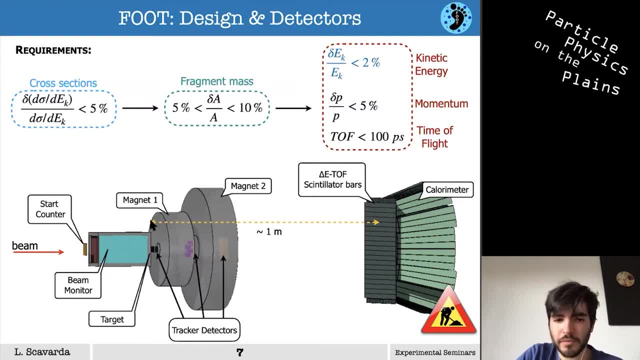 This experiment is little, As you can see. for example, the distance from the target and the calorimeter is about one meter. So the idea, indeed, of this experiment is to be a tabletop experiment. The idea is to move the experiment in different facilities. 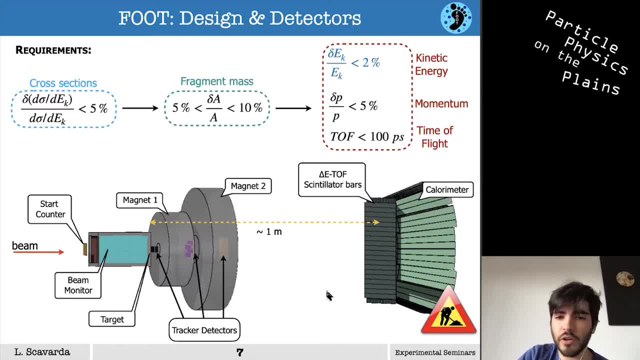 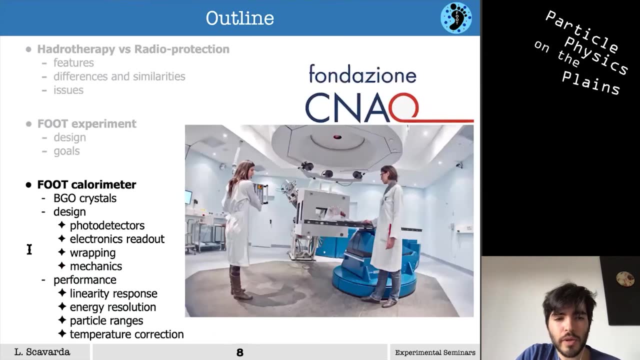 For example at GSA in Germany or at Knau in Pavia. I will speak better about Knau later And take data in different facilities with different beams. So now we can speak about the last part of my presentation, the biggest one about the calorimeter. 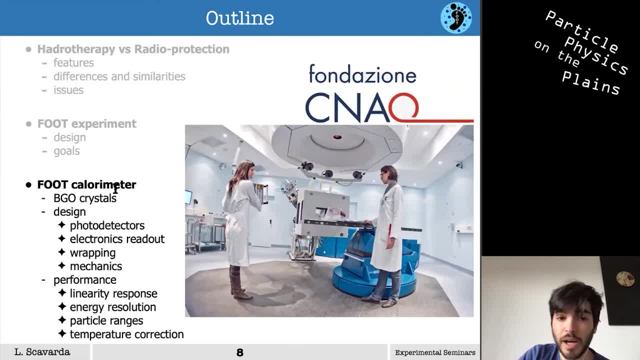 As I said, it's the main task of my group, So I will tell you about some test beams that were performed during the last years in order to make all the design choices for the calorimeter. The main requirements for the calorimeters, Of course, the linear response of the object, of the detector. 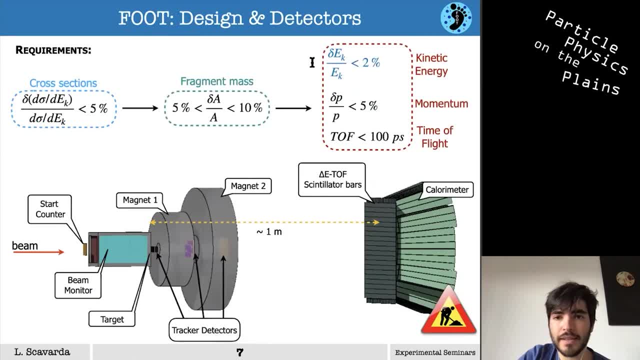 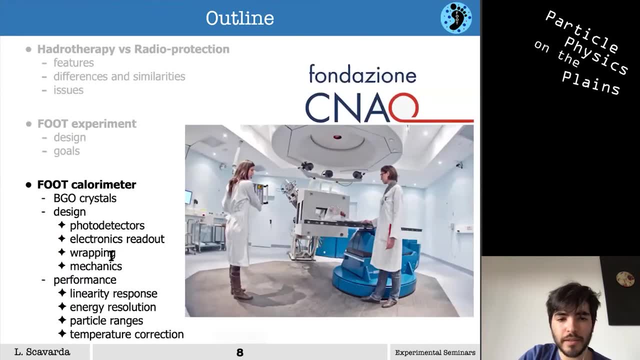 And the second thing is the kinetic energy resolution. We need a kinetic energy resolution below the 2%. So all the test beams that I will show you will be focused in order to obtain, to achieve this value. And the last part: I will show you some performances about the detector. 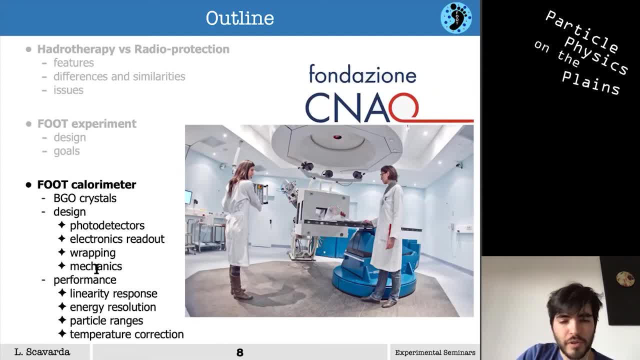 All the test beams that were performed during the last years in order to achieve this value. So all the test beams that we performed were at Knau, at Fondazione Knau. Knau is one of the most important centers in the world where they treat tumors with the adenotherapy. 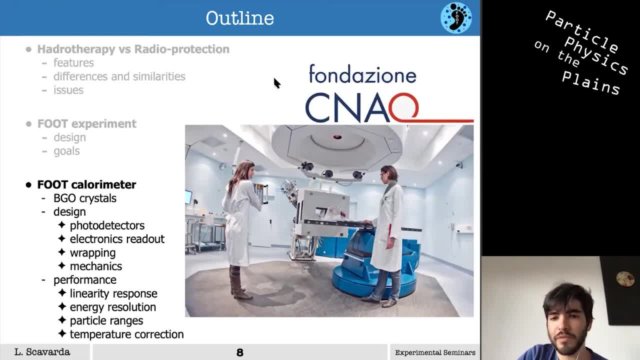 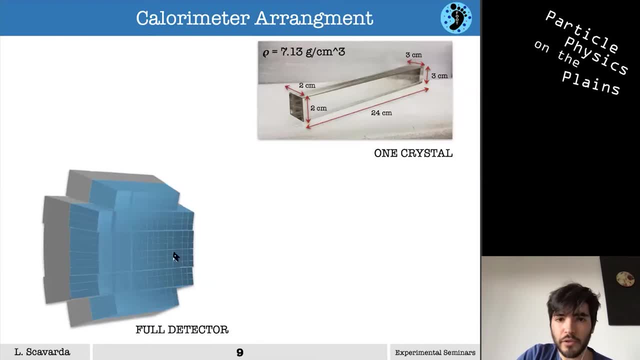 And this facility is in Pavia in Italy. Okay, we can start from the arrangement of the calorimeter. So, basically, our calorimeter is a measuring device. So, basically, our calorimeter is a measuring device And the detector is a matrix of Bee Geo crystals. 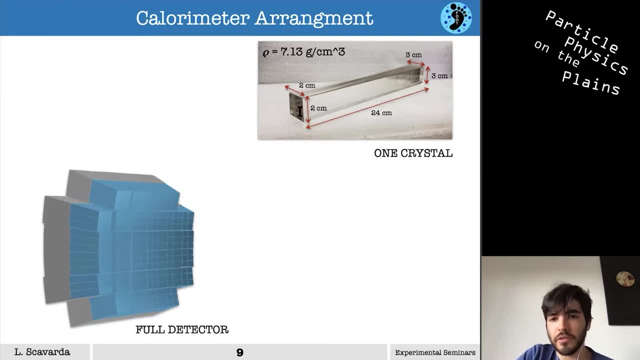 Here we have a picture of one Bee Geo crystal. As you can see is truncated pyramid And we have chosen Bee Geo because it has a very high density. So it means also very high stopping power And it means that we can stop a particle with higher energy also in few centimeters. 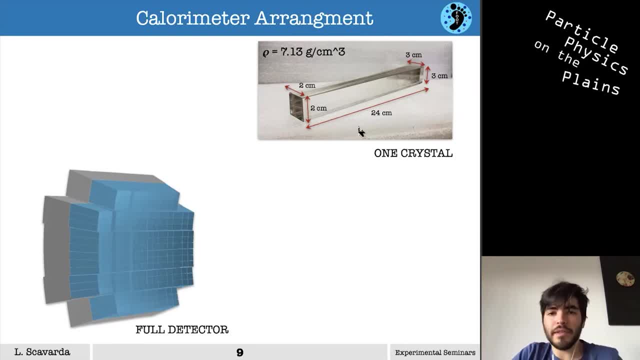 But the main problem with his object is the weight. is the weight because with this density, with this dimension, each crystal is about one kilogram. so it means that the full object is about 300 kilograms, more than 300 kilograms, because we'll have 320. 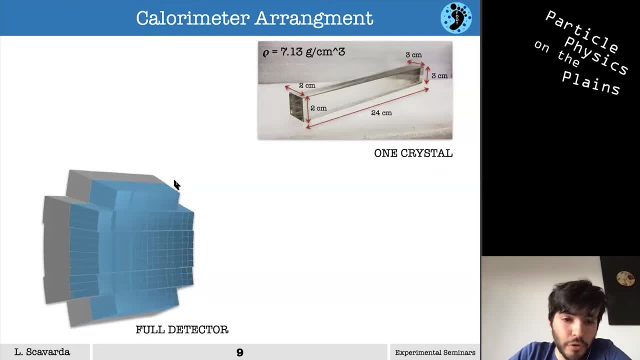 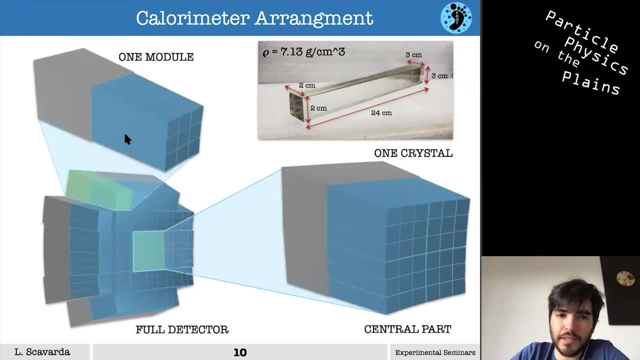 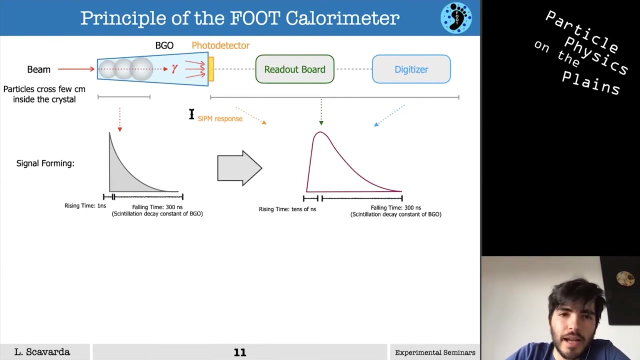 crystals. and the second problem is that we have to move it in different facilities. so the idea was to split all the detector in different substructures, called a module, where each module is composed by nine crystals, so only nine kilograms, okay. the calorimeter is a scintillating calorimeter, so it means that in order to know the energy of the initial particle, 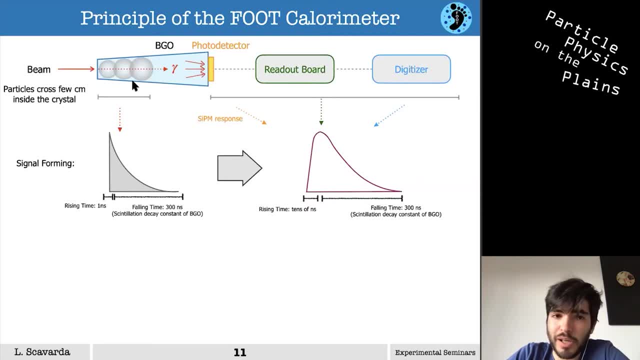 we have to collect all the photons created from this particle inside the video crystal by ionization process, so we can think, for example, to have a fragment or a particle beam that enters in the bgo and it loses its energy, so it creates photons, and we can collect photons with a photo detector. 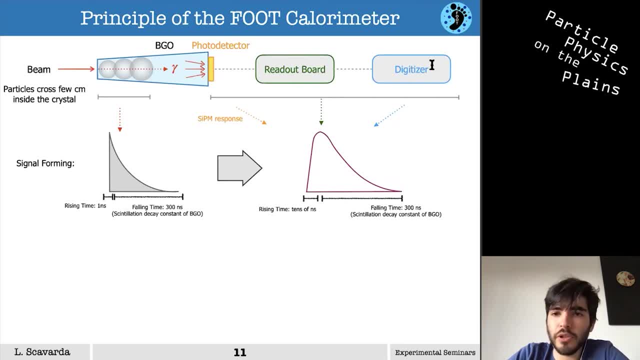 so then we can process it with the readout board digitizer, and we can. we can take the pulse, the pulse of the initial fragment. so from each pulse we can know two main information: the amplitude and the charge. the amplitude like the difference between the maximum amplitude and the pedestal, and the charge like the integral of. 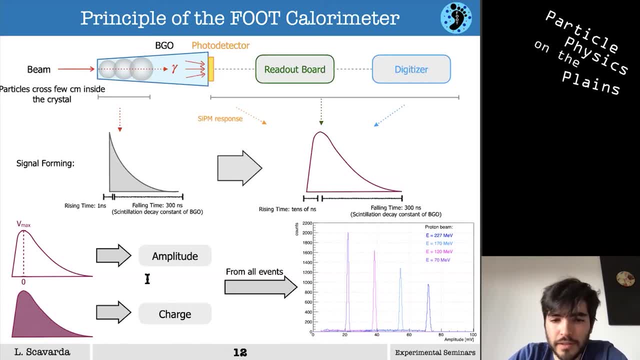 the pulse um. of course, these quantities are proportional to the initial energy. so what we have done in each test beam, in order to make all the design choices, was to, as i said, calculate the kinetic energy resolution and and the linear response of the calorimeter. So what we've done was shot. for example, 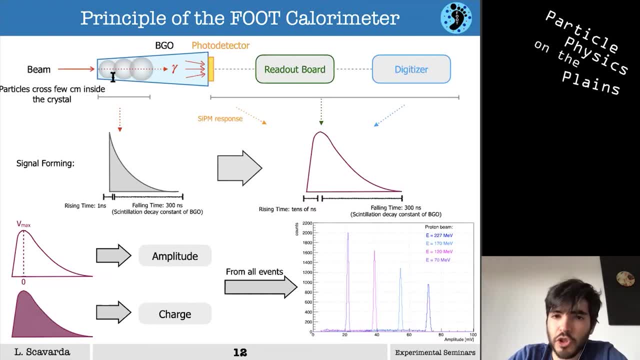 beams with unknown energy inside video crystals and calculate the amplitude or charge distributions for the specific energy, as you can see here, for all the events that we've acquired. So from each amplitude distribution or charge, we're performing the fit with a crystal ball function. 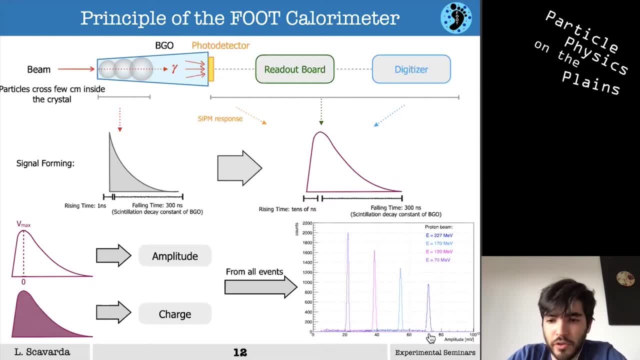 and we have extrapolate the average value, So the mean value of the Gaussian peak, representing the initial energy of the beam and also the energy resolution from the ratio between the width and the kinetic, and the average value of the peak. So the first test beam that I want to show you. 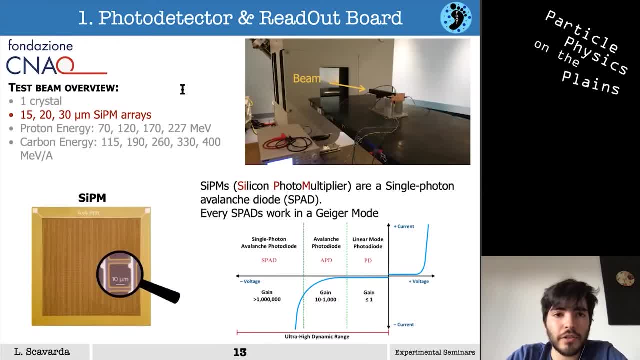 is the first test beam that we performed some years ago In order to choose the best photo detector for our purpose. So we have decided to work with the CPM. So John does some work about CPM. A CPM is a silicon photomultiplier. 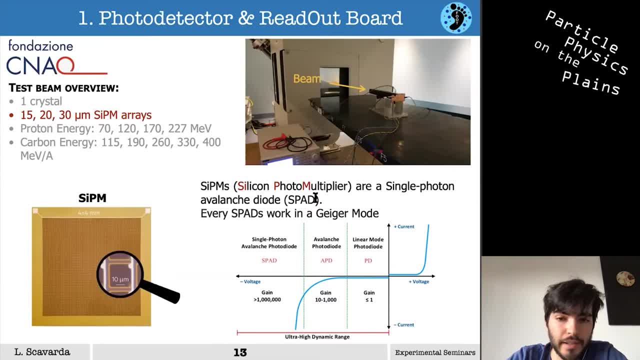 So it means a single photon avalanche diode like a SPAD, And it means that is a CPM is a matrix of these SPADs and where each SPAD works in a mode called Geiger, in a Geiger mode, So it means that the gain of each SPAD is very high. 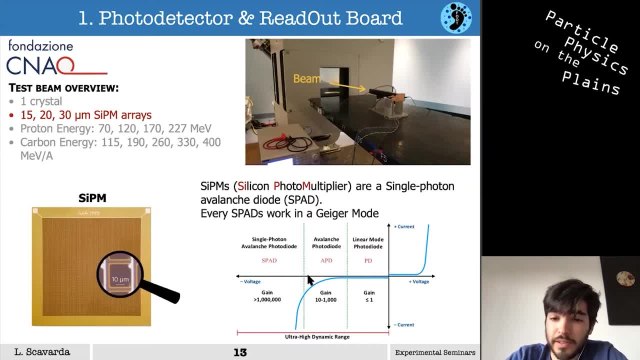 because the bias voltage applied to each microcell is really really high. So it means that each microcell can count only one photon in a specific time, in a specific interval. So this detector is really useful if you want to count photons, Because the number of photons will be the number. 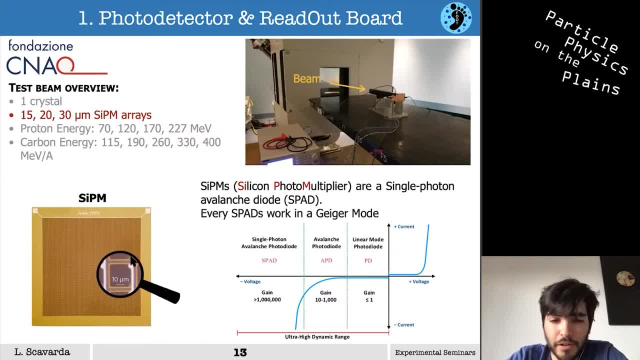 of the cells activated, the microcells activated, But there is a problem with this object, Because if you have more photons than the number of microcells, you will get a situation. So we have performed this test beam in order to understand which was the best silicon photomultipliers for our purpose. 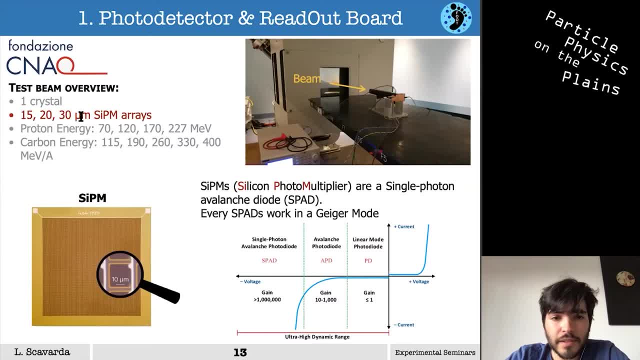 So we've tested different silicon photomultipliers with different the size of microcells in order to understand which was the best one, in order to cover the full energy range foreseen by the foot experiment. So what we have done was shot carbon and proton beams. 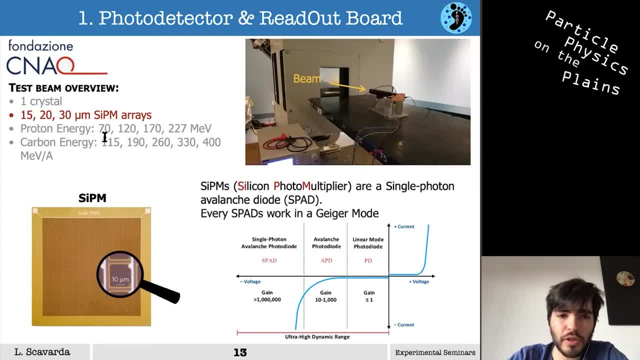 with these energies- four energies with proton and five energies with carbon- And. And then then we have measured the energy resolution and also the linearity response of the crystals for this energy. So here we have some results about this testing. In this plot we have the linear 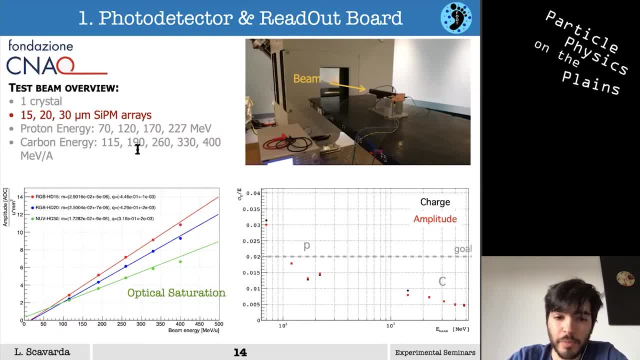 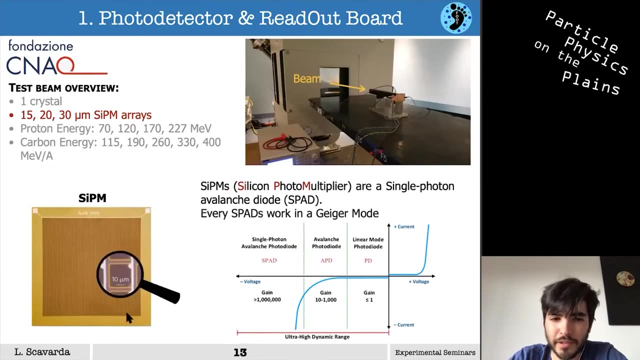 response only with the five energy of carbon beams for the three different silicon photomultipliers. I didn't tell you, but we are not using a single silicon photomultiplier like this, but we are using a matrix of this one, so what we call tiles. 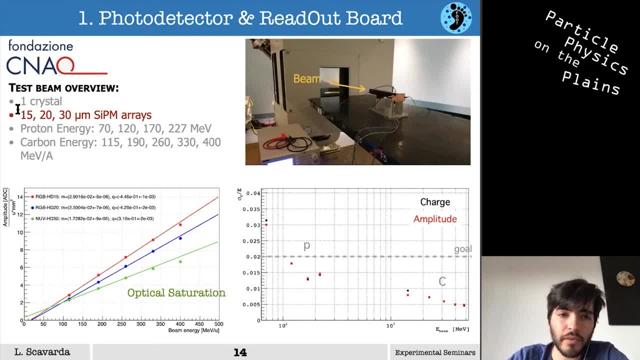 So in red we have the silicon photomultiplier arrays with 15 micrometers, in blue with 20 micrometers, so like the size of the microcells, and in green with 30. As you can see, with the, with the last one, with the green one, we have an optical saturation, So we've decided to work. 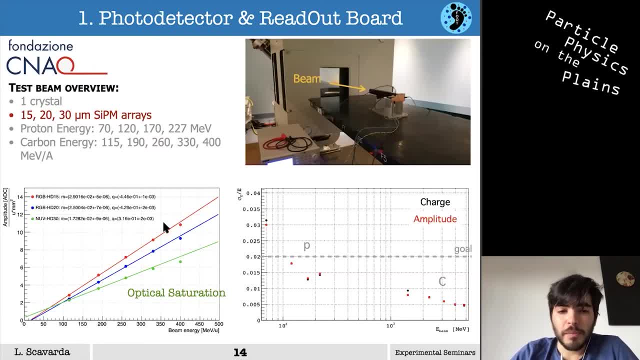 with the first one, with the 15 micrometer, because we can have also an extra safe factor if we want to extend the energy range of the beam up to 800 MeV per nucleus for the radio protections, for the radio protection measurements, In this case the points represent the average value of the 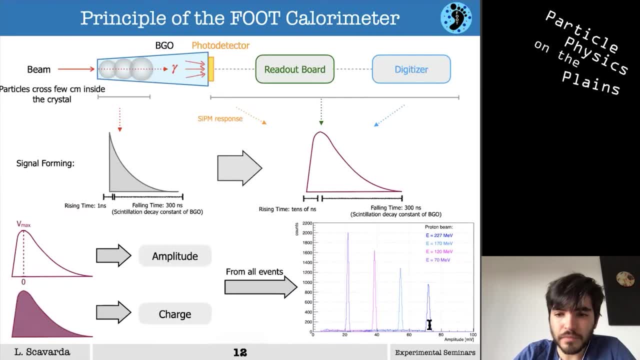 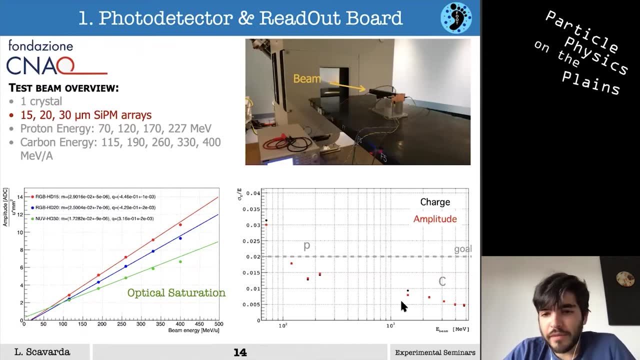 Gaussian peak that I showed you before here. So the linear response in terms of amplitude. in this case, On the right side, instead we have the, the plot related to the energy resolution. So, as I said, the ratio between the width and the average value of this Gaussian peak. 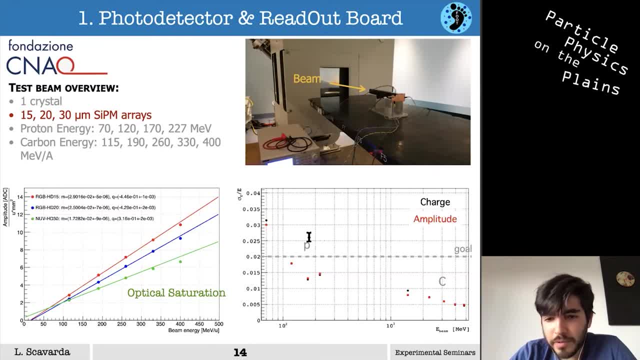 As you can see, here we have the points related to the carbon beams and here the points related to the proton beams. As you can see, we've got good results because, except for the lowest energy, we have achieved the energy resolution below two percent for all energies, And the different color represents the two different analysis that 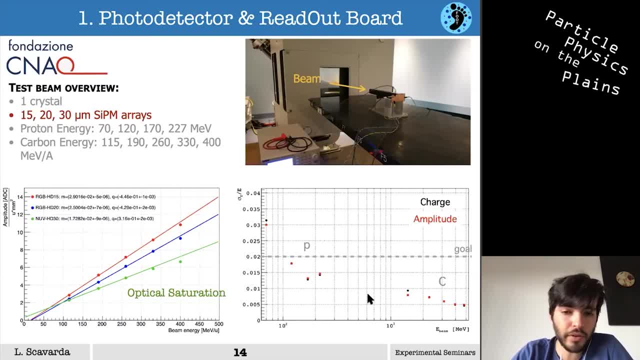 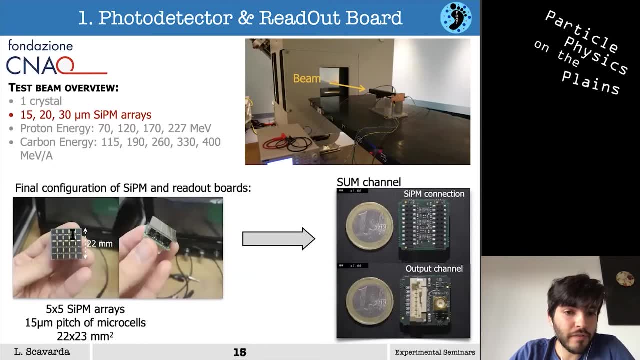 we've used, So in black the charge analysis, so the integral of the signals, in red instead the amplitude, And here we have a picture of the final configuration of the CPM and the readout volts. So in the experiment for the detector we will use a matrix of silicon photomultipliers, five by five, with a pitch as a. 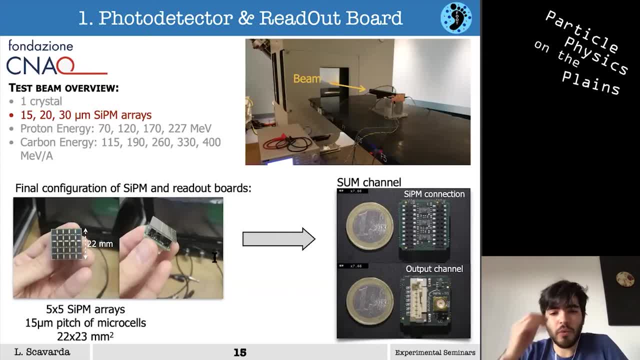 state of 15 micrometers with these dimensions. So we've decided to work with silicon photomultipliers because they are really small, as you can see from the picture, And so they can help us to have a really compact design. And the second thing was they work with a really low voltages. 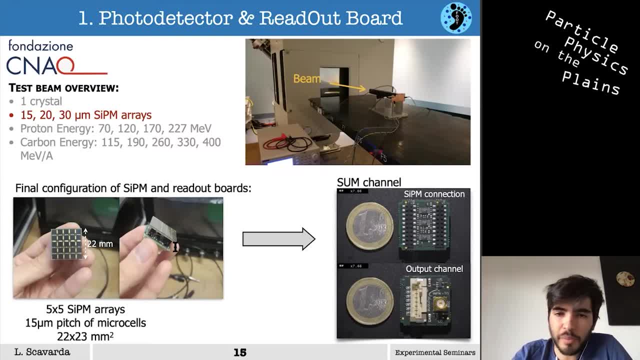 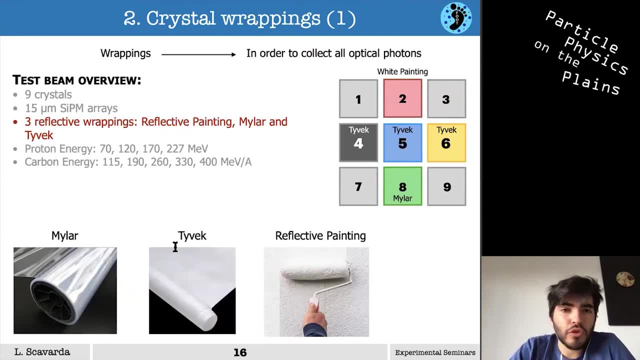 compared to other photodetectors like standard PMPs. Okay, the second test beam that we have performed was in order to choose the, the wrappings of the crystal, because thanks to the wrapping, we can collect as more photons we can. So in this test, 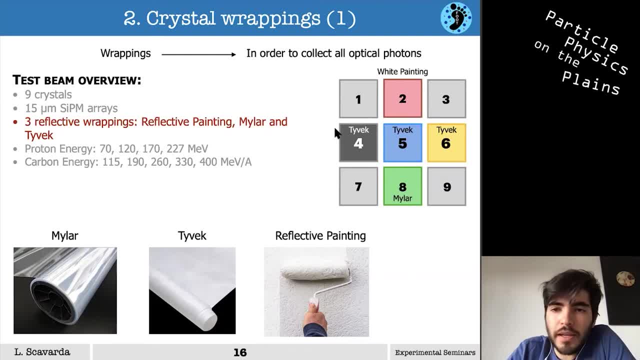 beam again at Knau. at Knau we use for the first time a module of the calorimeter, So nine crystals together, And we have equipped the different rows of the of this module with different kind of wrappings. In the first one we used a reflective painting, in the second one we used tyvek papers. 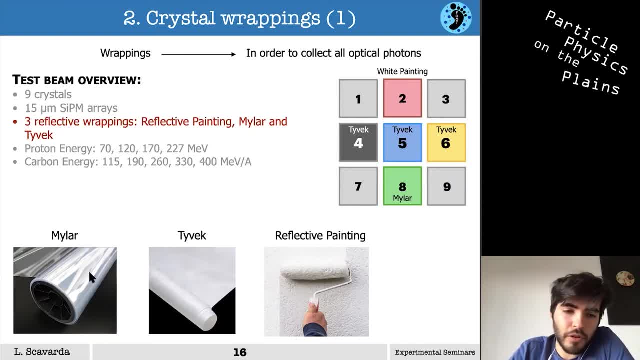 and in the last one a wrapping called Miler, a kind of aluminum. So again, what we've done. What we have done was shot the beam with the same energy used for the previous test beam. so the four energies for proton and five energies for carbon in the different crystals. 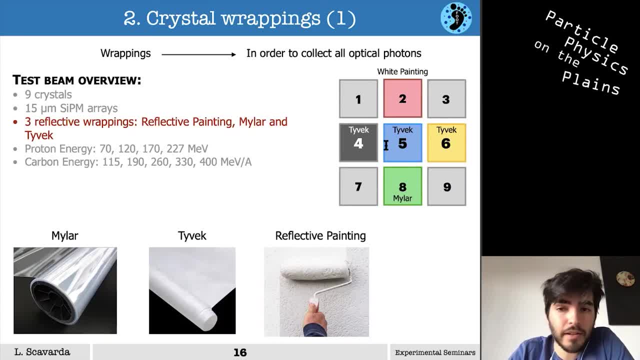 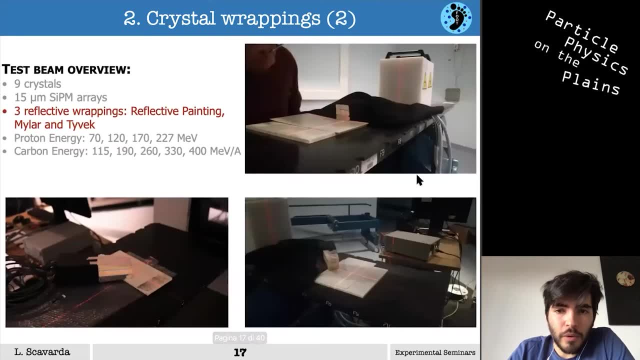 And we have again measured the kinetic energy resolution for each different energies and also the response of the crystal. Here we have some pictures about this test beam. Here we were in the treatment room of the canal. Here there is the treatment bed and here there is the model with the beam line with 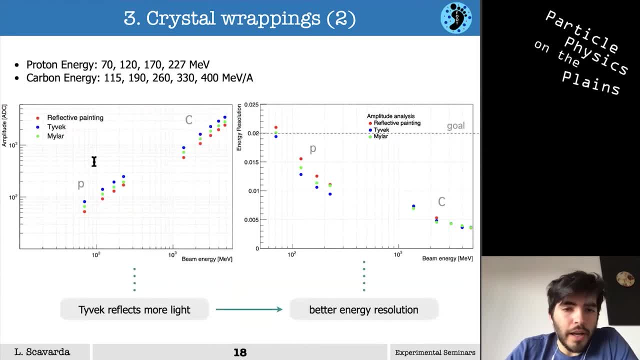 the laser of the beam line. Okay, in this slide we have some results about this test beam. On the left we have the plot related to the linear response, so the average value of the Gaussian peak calculated with the amplitude analysis. And here we have the linear response. 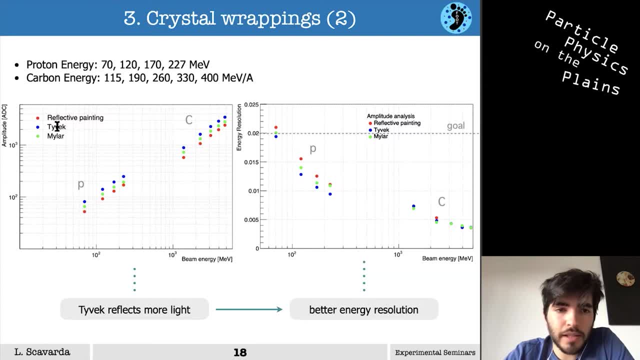 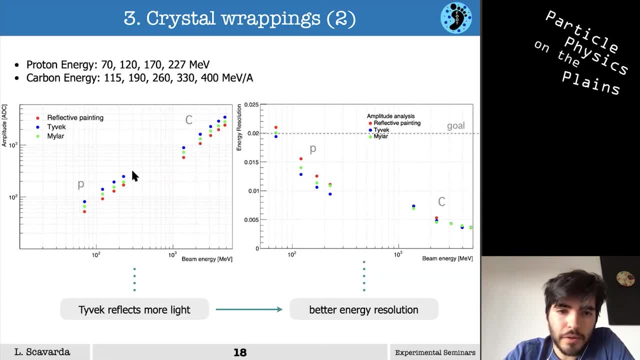 And, as you can see, with the tyvek, we can reflect more light inside the crystals and also it means collect more light And acquiring collecting more light, we can also obtain better energy resolutions. Okay, not much in the carbon, because they are pretty the same for all wrappings, but we have 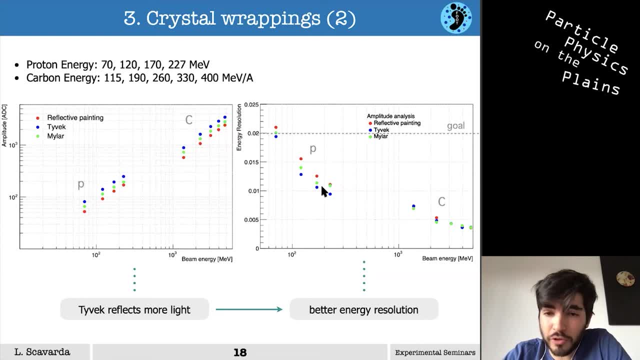 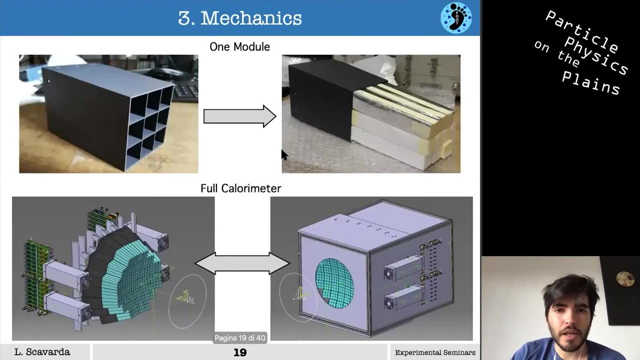 better resolution, in particular for the proton energies, so for the lower energies. So we decided a second point for the design of our detectors: the wrappings after the photodetector. Okay, in this slide I wanted to show you some pictures about the mechanics. 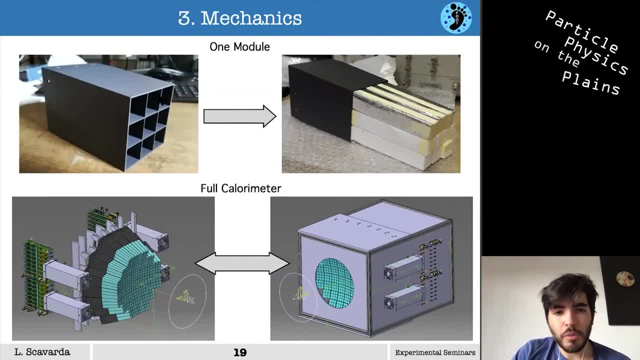 Here we have an older related to one single model. Basically it's a single model. It's a box with nine holes, so one for each crystal. Instead, here we have the idea of the full color meters. As you can see, we have all the models and the structure to all the models and also the HV and low V voltage. related to the voltages, 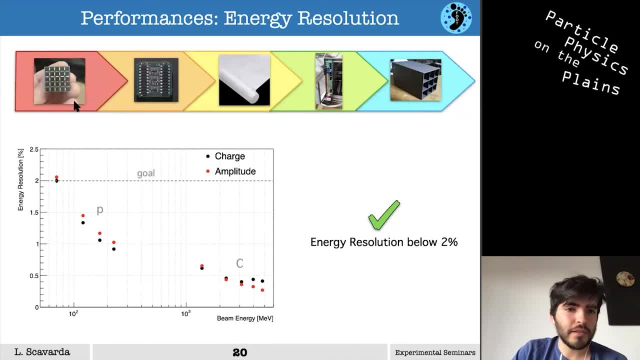 So, thanks to all these parts, these pieces, we have made all the designs, The design choices for our color meter, the silicon photomultiplier, the readout board with the same dimension of the silicon photomultiplier, So the design is really compact- the wrappings, the ADC, the digitizer. 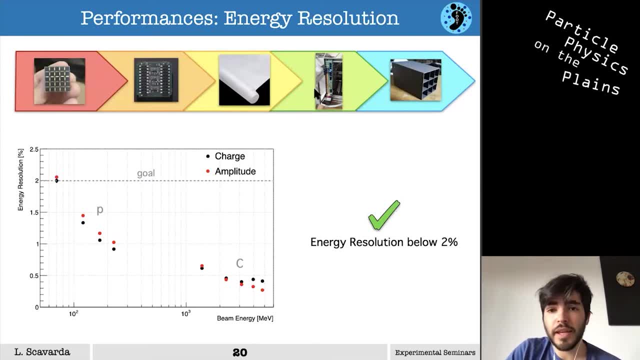 I didn't say anything about this, but we have performed a lot of tests about the digitizer in order to understand if we wanted to do pulse shape analysis or not, And finally, the mechanics. With all this in mind, we are now ready to go. 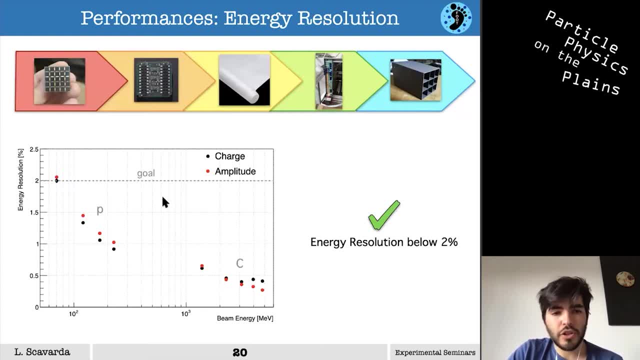 With all this information we have achieved our goal. So, in the full energy range foreseen by the experiment, the energy resolution below the two percent. And here again we have the double markers, one calculated with the amplitude analysis and the second one with the charge analysis. 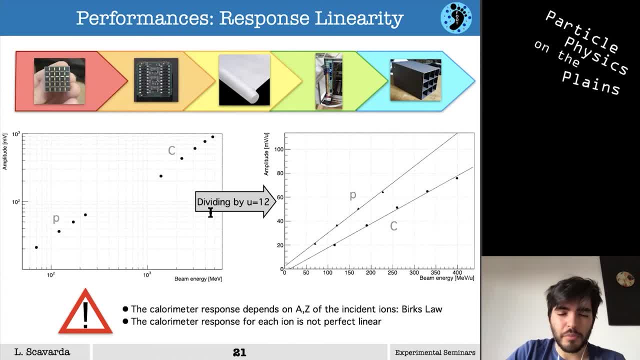 OK, about the linear response, we have some issues because here we have the, The average value related to the amplitude distribution for the carbon beams and here for the proton beams. So dividing these points by the mass number of the carbon in order to compare better the two trends, we can see there is a problem because the response of the colorimeter depends on the A and zeta of the incident ions due to the Birks law. 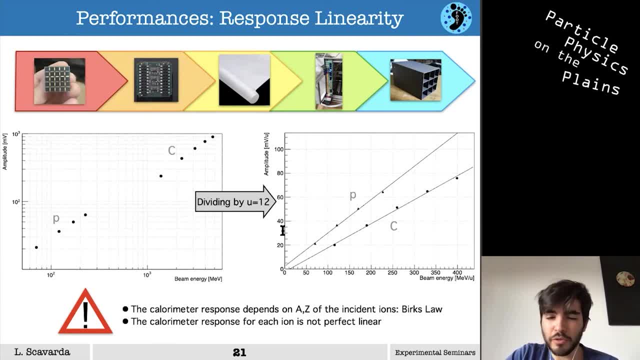 So it's a problem because from a certain amplitude or charge, we can't know the initial energy of the fragments, because for for a specific value, we have two values in energy. So it's a it's a big problem but we think that for this we can't do anything. but we can solve this problem thanks to the other detectors input, for example, from the detector in front of us, the top wall. 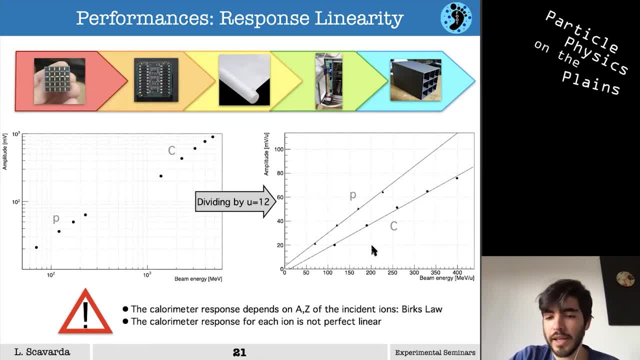 The plashing plastic And the top wall is the top wall of the shingletor, because the top wall can give us the zeta of the particle from the energy loss in the shingletor bars, so from the zeta of the particle. in principle we could distinguish between different ions. 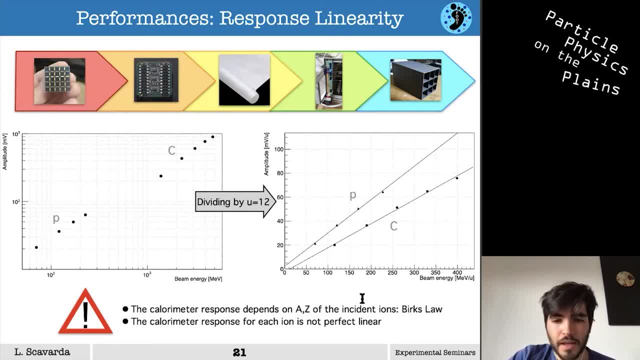 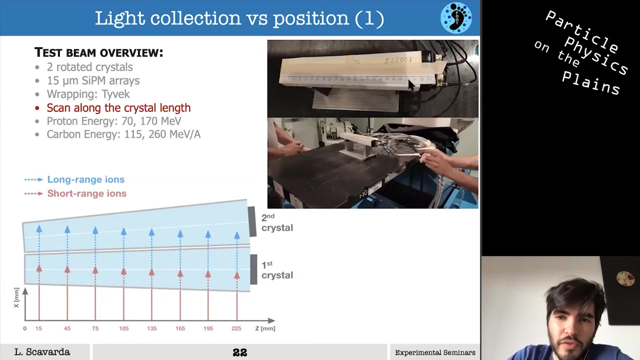 But more tests will do it in for this study. and the second thing is the. the colorimeter response for each different ion is not perfectly linear, in particular if you look the carbon points. So if we want to understand better this, This thing, we have performed another testing at now, and this time we've placed to be Joe crystals rotated by 90 degrees compared to the beam line. 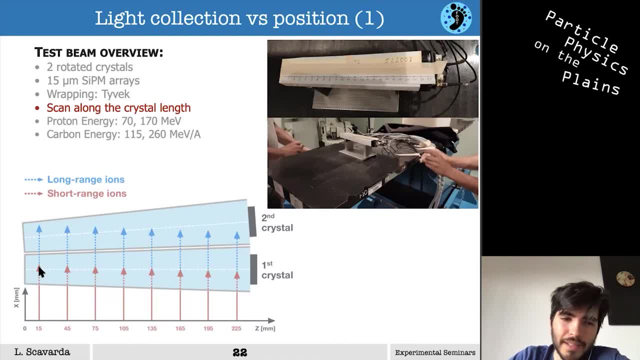 of now, and so we perform it: a scan with the beam along the length of the crystal, Three centimeter by three centimeters in 15 millimeter, so in the fastest point from the silicon photomultiplier up to 215 millimeter. so very close to the silicon photomultiplier. and why this? because we wanted to. 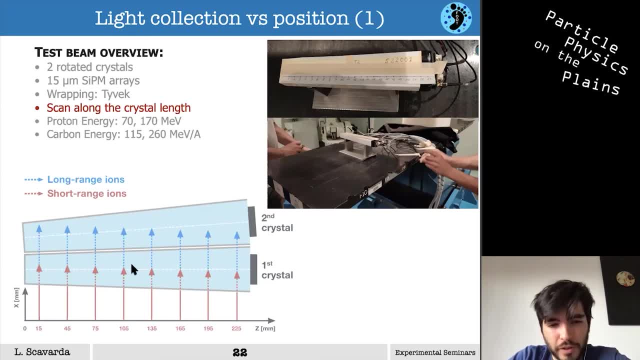 understand if the response of the crystals depending or not with the depth of the particle inside the video crystal. so we use two beams again, proton and carbon, but only for energies: 70 MeV for proton and 150 MeV per nucleon with carbon in order to have the black peak inside. 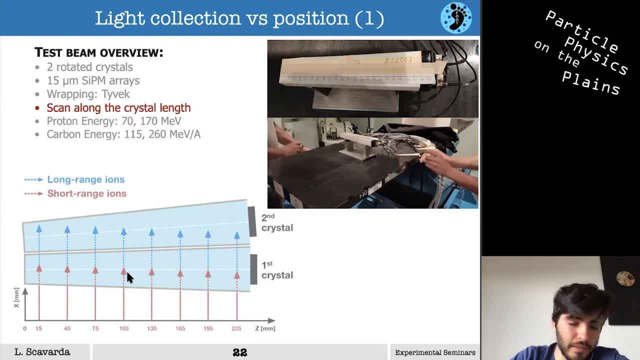 the first crystal. so, in order to contain the the full range of the particle inside the first crystal, with 170 MeV and 260 MeV per nucleons instead, in order to have the particle inside the second crystal for this case. so we have summed up the light with sum up the light in the two crystals. 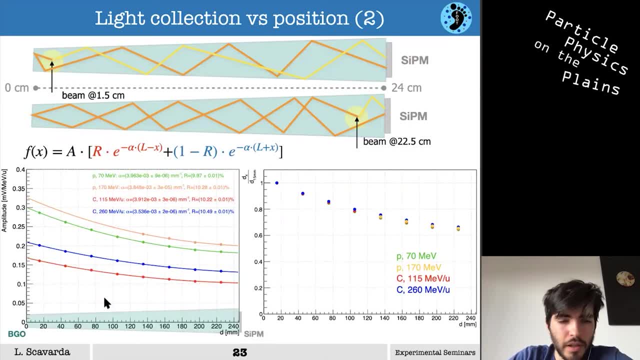 okay, here we have the results about this test spin. so we can see that with different colors, with the different particles and energies, for example, in red we have the scan with the carbon 115 MeV per nucleons and we can see that the light collected is not constant. but 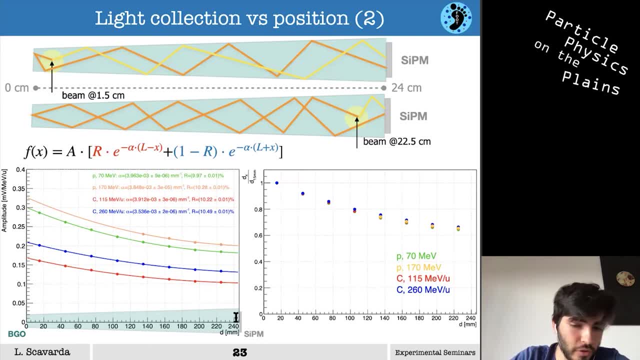 more we are closed, closer to the cpm, less light we have collected. so the results was a little bit unexpected because we thought a constant response, or at least the opposite trend: when we are closer to the cpm we we could collect more light. So first of all we've tried to understand if this 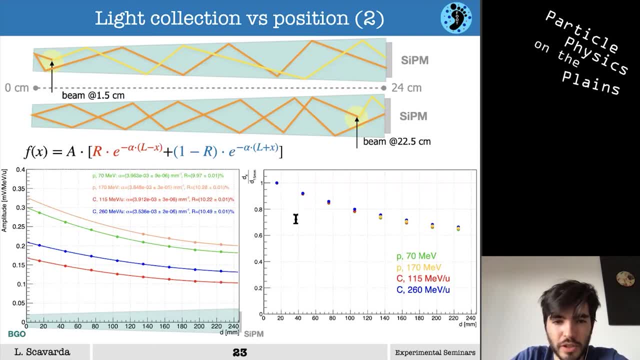 effect doesn't depend on particle and energies. So in this plot on the right side you have the ratio between the amplitude, or the charge of course, acquired in the different position, normalized to the amplitude in the fourth position. So I just normalize all the points with the first one And, as you can see, 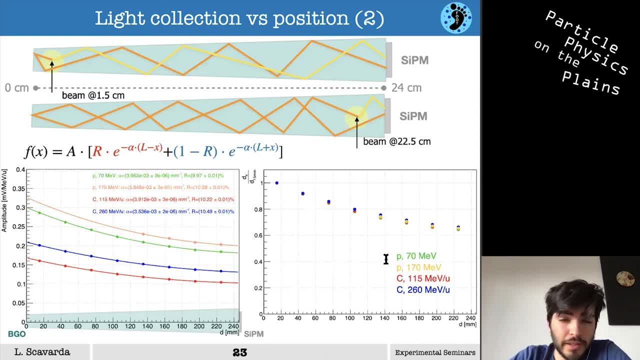 this effect is the same for all particles and energies, So at least this effect doesn't depend from the network part. One hypothesis about these that we thought was that, for example, if we imagine to have been here so very far to the CPM, we can imagine that the 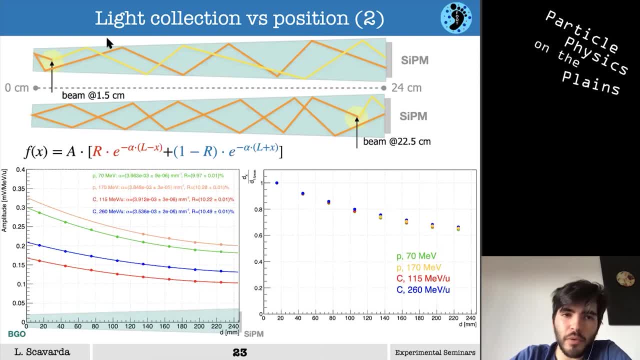 light is divided into components, one directly to the CPM and the other one go to the opposite side. But the problem is when we are here, when the first component, directly to the CPM, is reallyédirected to the light and the first component is not. 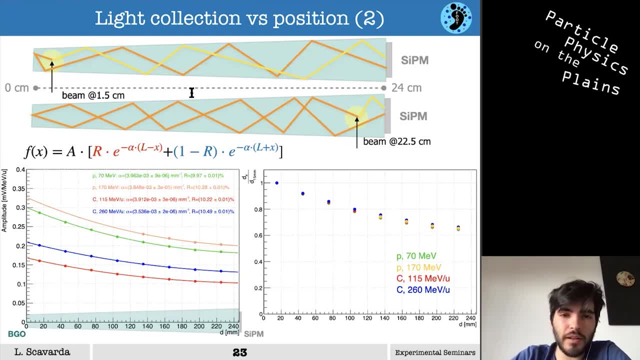 right, And so if we have the beam here, when the first component directs, the CPM is really short, but the other is has to do almost the double of the length of the crystals, and so it has to do much more. reflections respect the first point. 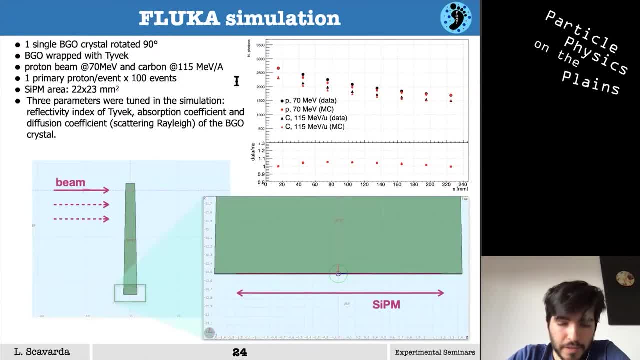 In order to investigate better this, this effect, I performed some Monte Carlo simulation, in particular with the Fluca, with the Fluca software. so what I did was simulate and create the geometry that we use that now, this time only with a single crystal and not with two. 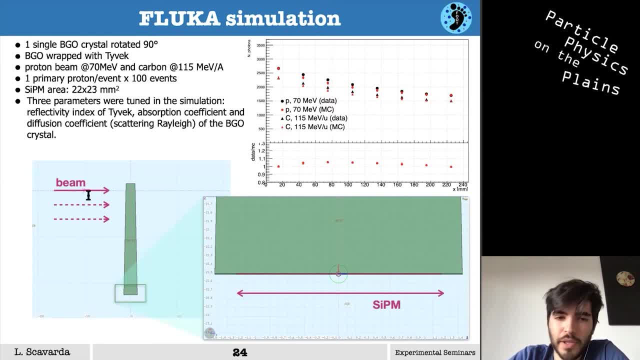 crystals, but again rotated by 90 degree compared to the beam line, and I simulated the beam position, the same that I use that now. The core of the simulation was the tuning of three different parameters and first of all the wrappings of the crystals, so the reflective image. 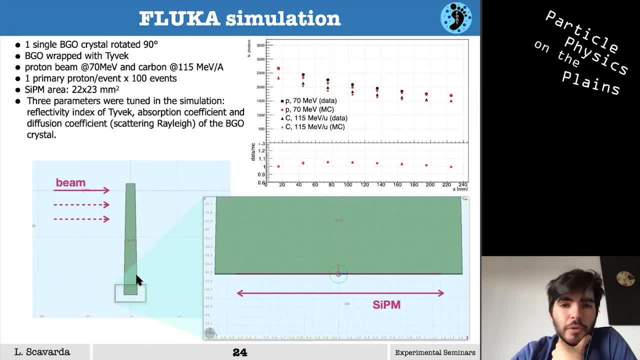 index of the Tyvek, and then also the absorption coefficient and diffusion coefficient of the video crystal. So after a fine tune of this tuning of these parameters, I found the best one that can allow me to get a good agreement between that and Monte Carlo. As you can see from this plot, 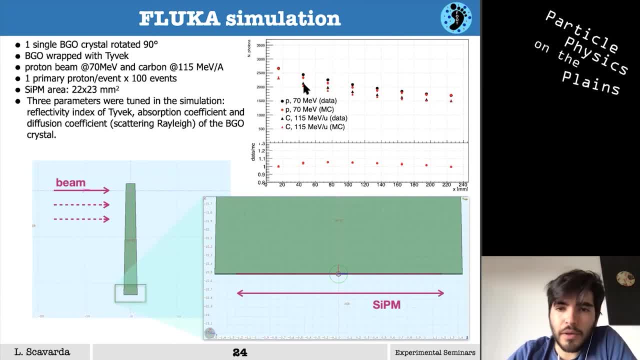 in black we have the data acquired up now, in with the circle for the 70 MeV, with the triangles for the 150 MeV per nucleus carbon, and in red we have the Monte Carlo simulations, so we can see that the agreement is within the five percent. Ah, yes, I simulated also the silicon photomultipliers, but only as a. 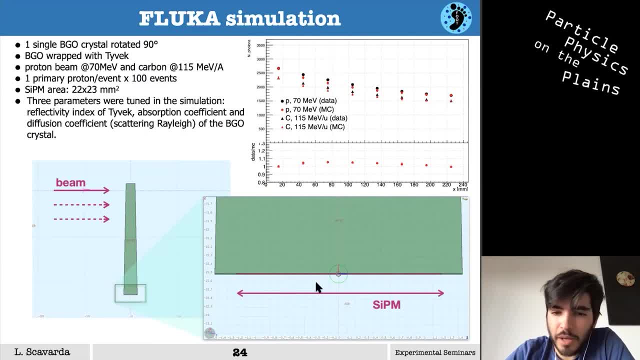 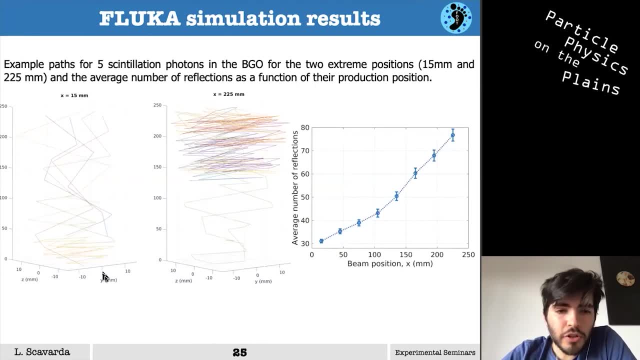 active area inside the BGO. in order to count the number of photons collected in this area for the different beam positions From the simulation, I also calculated the number of reflections inside the video crystals, For example. in this slide we have an example of path for five scintillation photons in the two 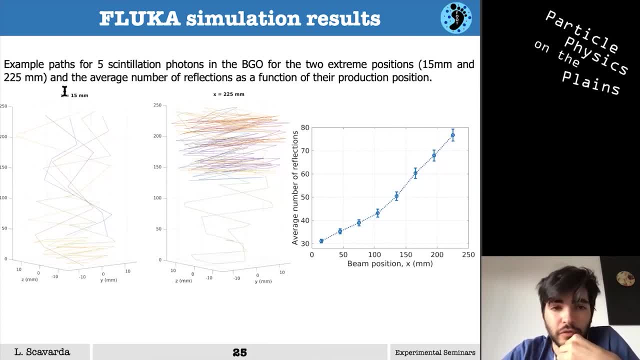 extreme positions, So in the fastest position from the CPM in 15 millimeter and in the closest position, so in 225 millimeter. As you can see, the reflections here are much more respect compared to the, the first position and also the other positions, And this is confirmed also in this plot where we have the number or 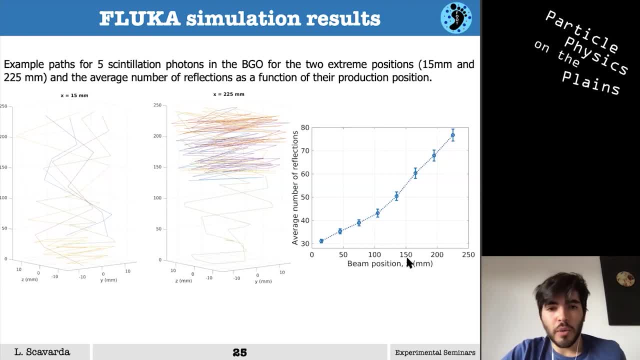 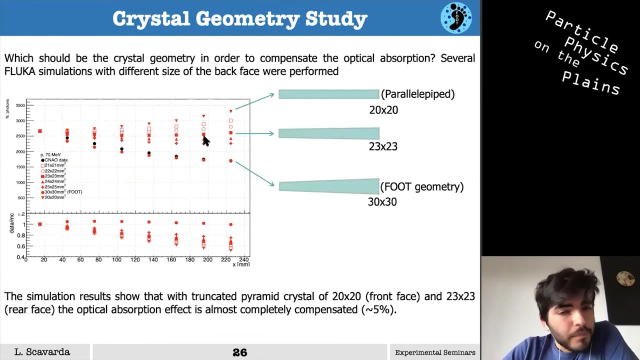 average number of reflections versus the beam positions. So our hypothesis was true. So if we have more reflections, also the probability to be absorbed inside the BGO is much more higher. Okay, So, um, what I did after this was to understand, because this problem is also related to the 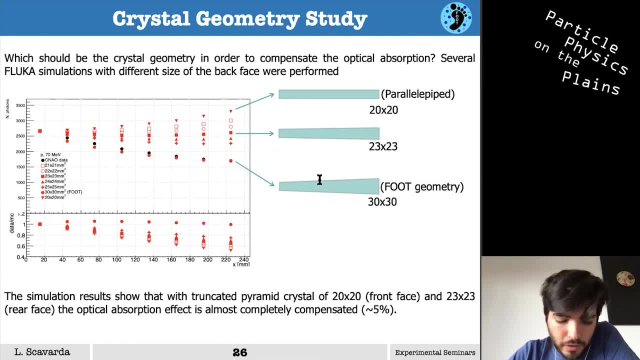 geometry of the crystal. So I tried to understand if there was a geometry of the crystal in order to compensate this effect. So I simulated again this, this effect, with different geometry of the video crystals. So here we have the standard one, the, the BGO that we have in foot. 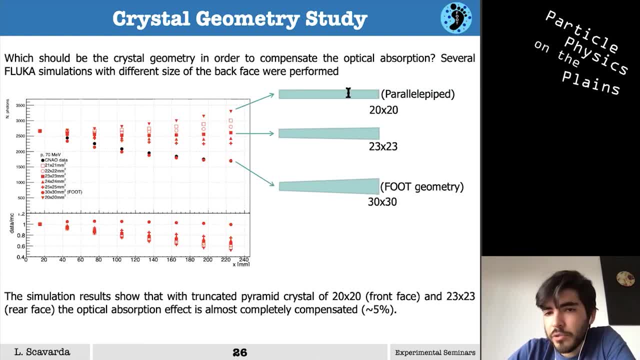 And I changed the rear face of the crystals up to an extreme case with a parallelepiped. So I found that with a truncated pyramid with a rear face of 23 by 23 millimeter square, we can have a constant, a constant light collected. So with this geometry we can compensate. 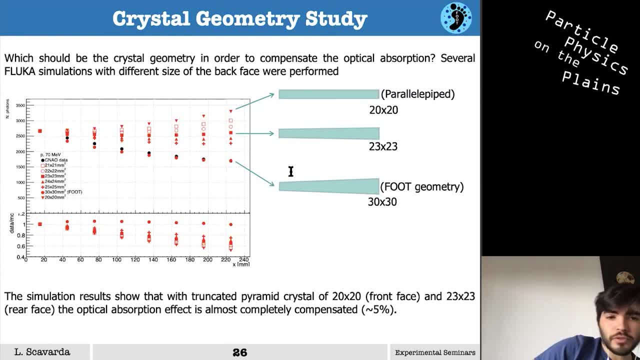 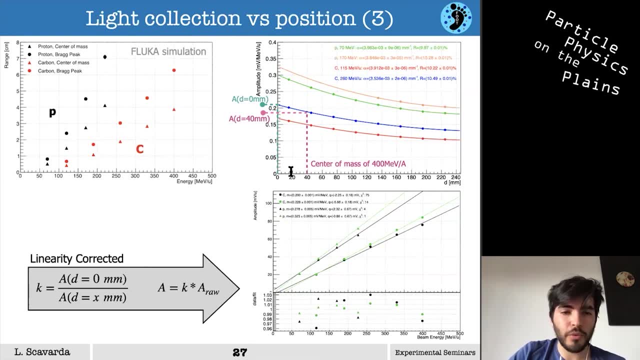 within a fiber percent, the, the absorption inside the video. But anyway, we have this problem inside the video crystals. We have this BGO. We don't have time to modify the geometry, cut the crystals etc. So we need to compensate this effect offline with some correction method. 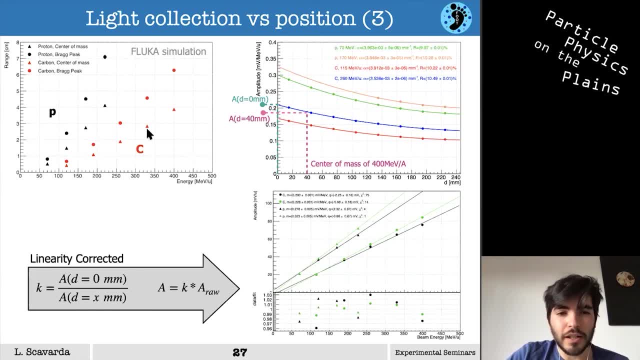 So I performed other fluke simulations and I performed in in this time simulation in order to know the range of the particle inside the video crystal. So here you can see the the position of the range, So the Bragg peak of the particle inside the BGO. 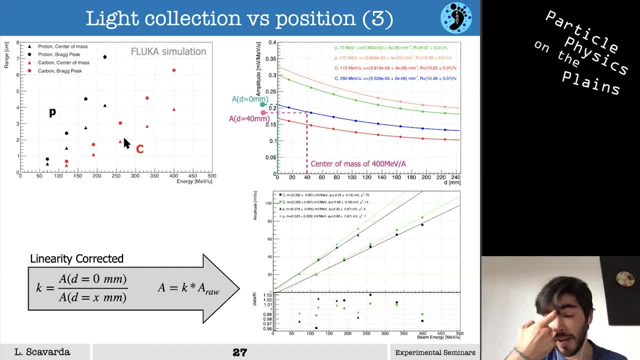 for the car, for the five standard, for the five standard energy used up now. And here the four position, the position of the Bragg peak for the energy of proton used again. now With the triangles instead we don't have the position of the Bragg peak, but let's say the center of mass, if you will. 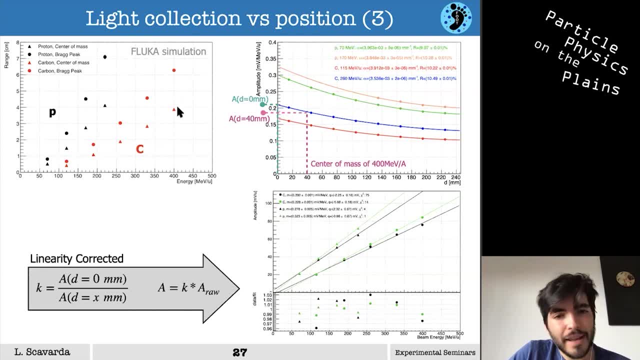 if you want, like an average, average distance of the emission of the photons, because we know that of course the most part of the photons are emitted in Bragg peak, but we can assume that some photos are emitted also before. So we have also the position of the 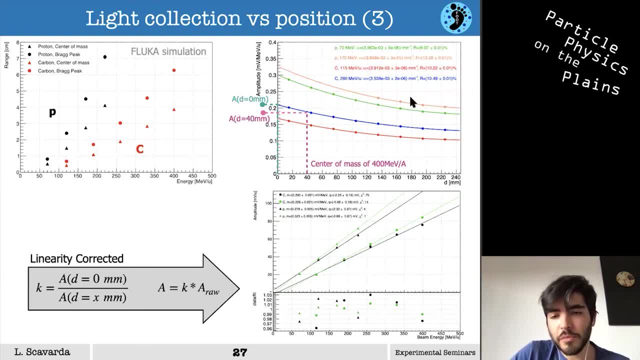 center of mass. Okay, From these plots we can calculate the correction for our linear response. So, for example, we can. we can take one particle like carbon with 400 mm per nucleon and we can know directly that it's range of the center of mass is four centimeter. 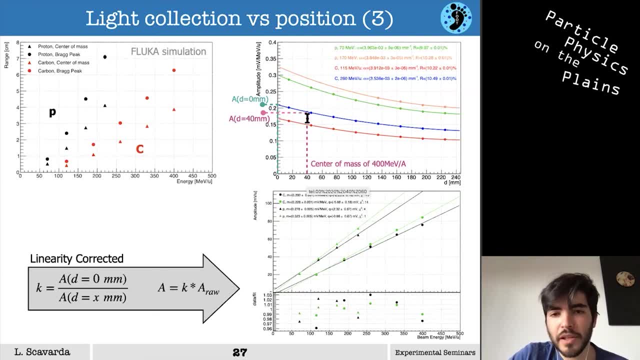 So from this four centimeter or 40 millimeters, we can know directly the amplitude, so the light that we collect with the average amplitude, so the average photons that we can collect with this energy. Of course we can use one of these trends because we have seen that the 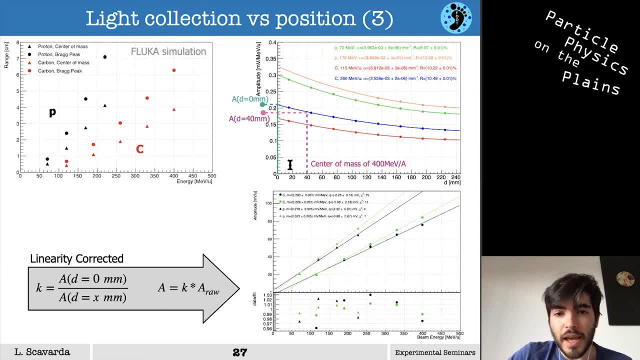 effect doesn't depend from particle and energies, And also we can take the amplitude if this effect would be not present. So if the particle crosses zero millimeter inside the video crystal, From the ratio between these two values we can find the k factor. in order. 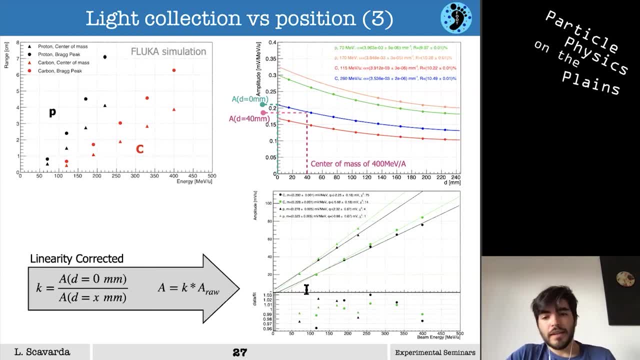 to correct the amplitude. So in here we have the linear response of the calorimeter after the correction. so after this formula, In black we have the band before and in green we have after the correction, as you can see both from the chi square. 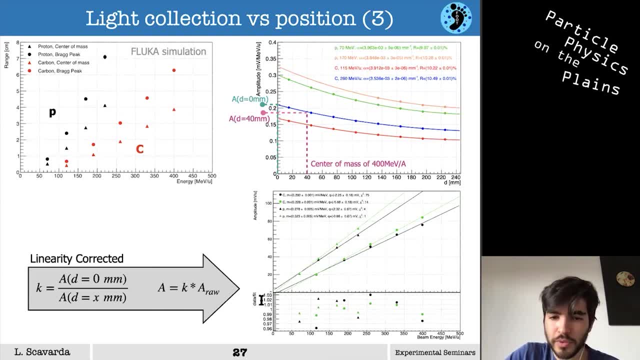 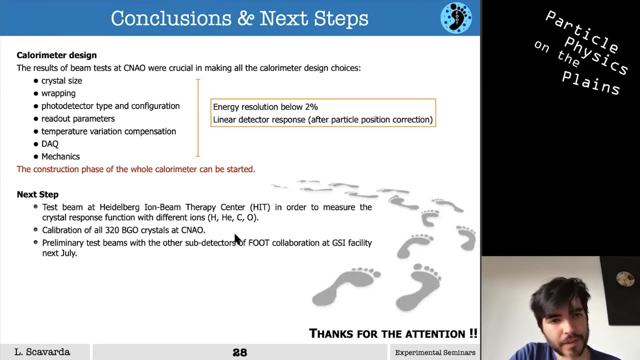 of linear fit. on this points, but also from the ratio between data and evaluation of the fit, we have improved a lot. the linearity response Ok. in conclusion, all the results of the test we made now were crucial in making all the final results. 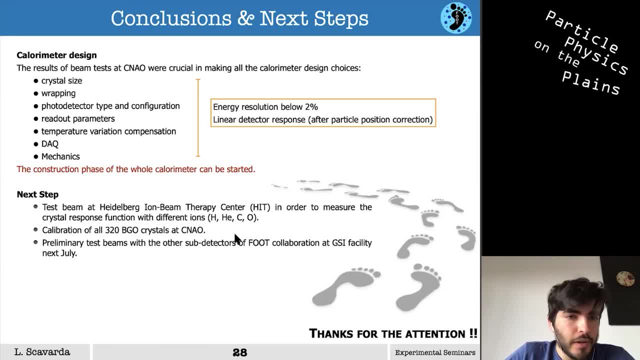 calorimeter design choices, As I said, about the crystal size, the wrapping, the photo detector type and configuration, the relative parameters. I didn't speak about temperature variation compensation, but I have also some information, the backup slide, if there is time about this. 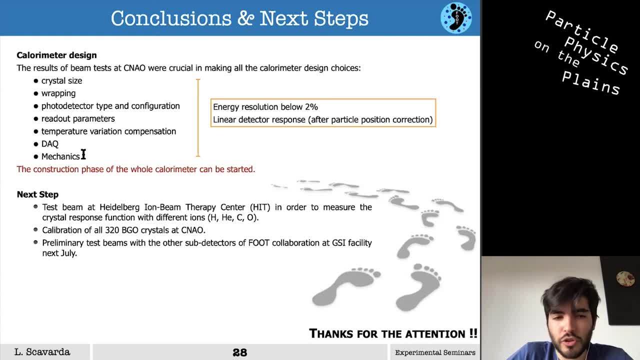 study the DAQ, that I didn't show you anything, I'm sorry, and also for the mechanics. With all this information, we have achieved our goal in terms of energy resolution And we have obtained also a good linear response in the. 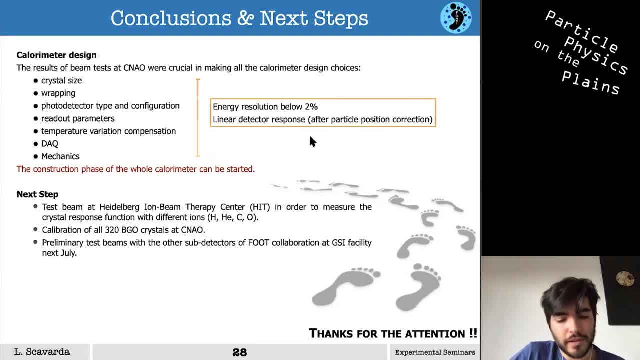 chlorimeter, of course after the particle position. There is still the problem about the Birch's law, about the response for different ions, but for this in the future there is planning At a test beam at the Heidelberg ion beam therapy center in order. 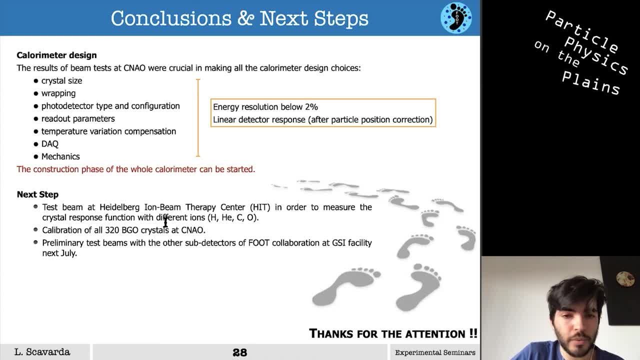 to measure the crystal response function with different ions, with the hydrogen, helium, carbon and oxygen, So in a facility where we can have a lot of sources. Then also in the future, in the next month we will calibrate, we will proceed with the calibration of all the 320 Bijou crystals up.